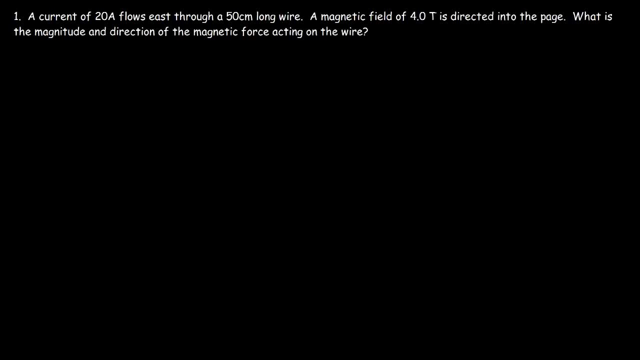 A current of 20 amps flows east through a 50 centimeter long wire, A magnetic field of 4 Tesla is directed into the page. What is the magnitude and direction of the magnetic force acting on the wire? So let's draw a picture. So let's say if we have a wire or even a conductor. 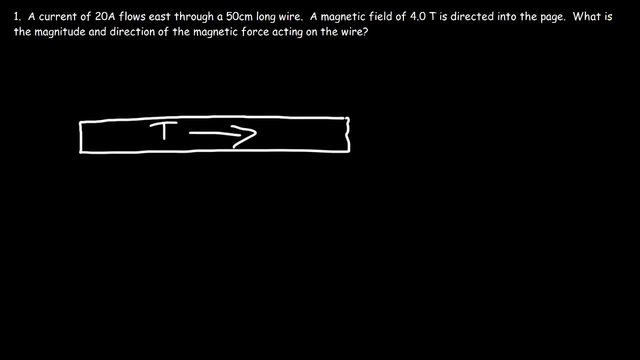 and there's a current flowing east in that direction, And so we know the current is 20 amps. Now the length of the wire, it's 50 centimeters long. How can we calculate the magnitude and the direction of the magnetic force? Now the magnetic field is directed into the page, So we can use a. 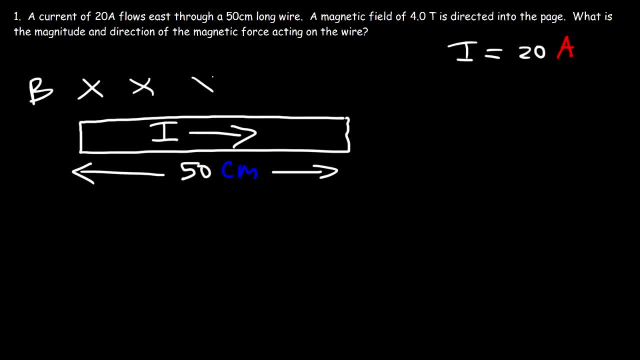 symbol of X to represent that. So everywhere is directed into the page. And the strength of the magnetic field? it has a magnitude of 4 times Tesla. so calculate the magnitude and direction of the magnetic force. let's talk about the direction, and so we could use the right hand rule if you stretch. 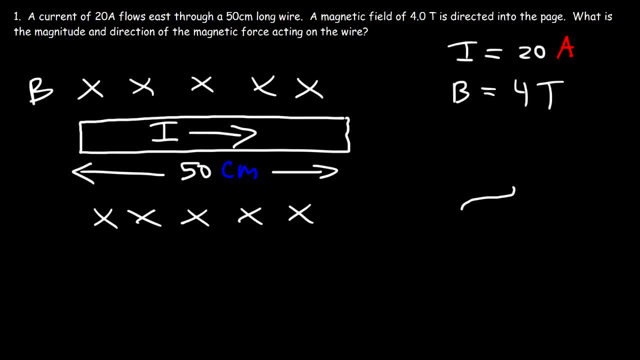 out your hand like this: direct your thumb in a direction of the current and the four fingers you need to point it into the page. so if you draw your hand like this, this is the direction of the current, it's going in the positive X direction and the fingers, your other four fingers, are directed into the page and then out. 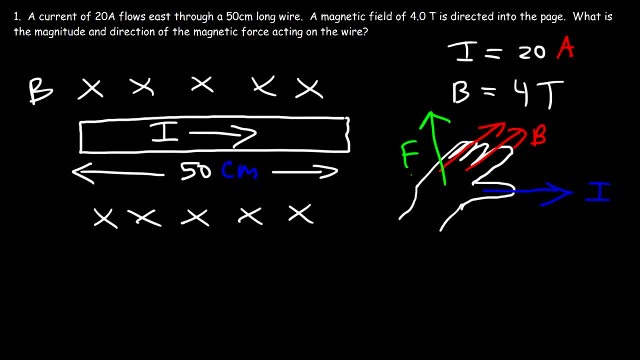 of the palm of your hand, you should have the magnetic force which is directed north. so hopefully you can see it based on the drawing. but if you direct your four fingers into the page and the thumb east- the force which comes out of your hand- you should see the palm of your hand facing north and so that's the direction of the. 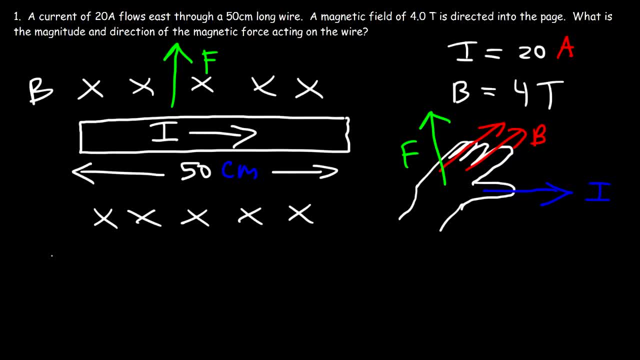 magnetic force acting on the wire. now let's calculate the magnitude of the magnetic force, and the formula that you need to get the answer is this equation: it's equal to the current times, the length of the wire, times the strength of the magnetic field, multiplied by sine theta and theta, the angle between the magnetic field and the. 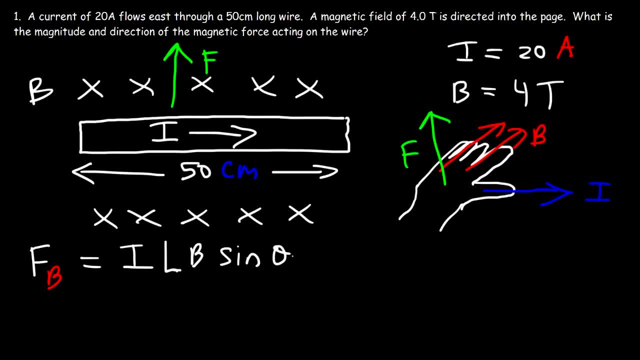 current, or basically the length of the wire which is moving in a direction of the current. so the current is moving in this direction and the magnetic field is directed into the page. now these two are at right angles: the current is x-axis, or positive x-direction, and the magnetic field is going into the page. so 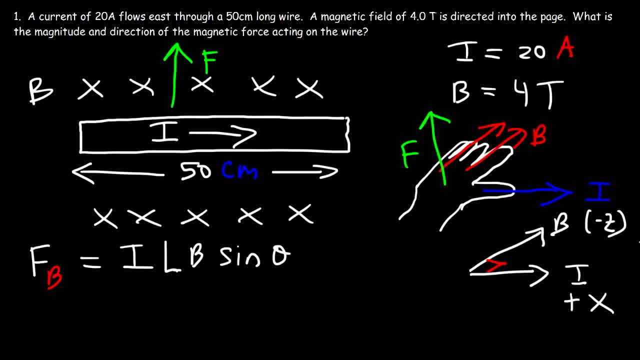 that's going to be in the negative z-direction. So, even though this doesn't look like a 90-degree angle, if you can draw correctly it really is. So let's say: if this is the positive x-direction, this is positive y, and let's say this is the 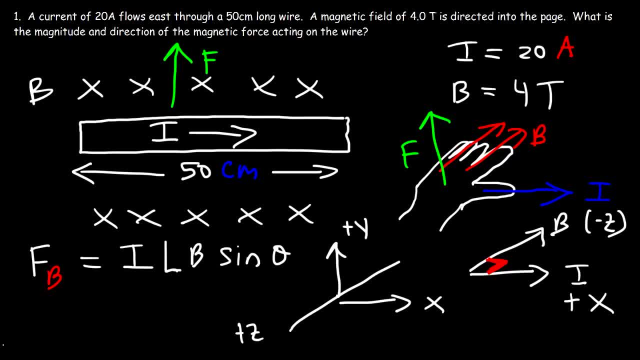 z-direction, Let's call this positive z. So in this case, here is the magnetic field and the current is in this direction And this is the angle between them. So we have a 90-degree angle and sine 90 is 1.. So in this example, the 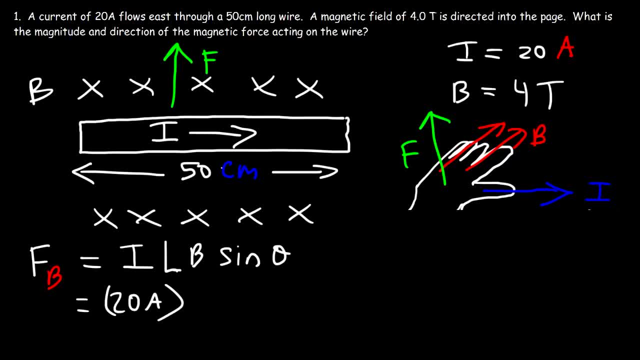 current is 20 amps. the left of the wire is 50 centimeters, but we need to divide that by 100 to change it to meters. So 50 divided by 100 is 0.5 meters and the magnetic field is 4 Tesla multiplied by sine. 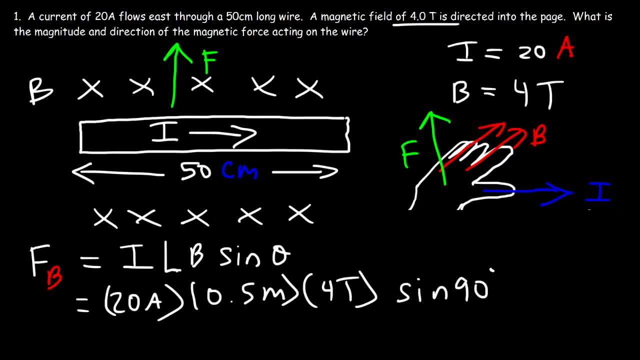 of 90 degrees. So 20 times 0.5 is 10, and 10 times 4 is 40.. So the magnetic force is going to be 40 Newtons, And so that's the magnitude of the magnetic force and the direction it's pointed north. 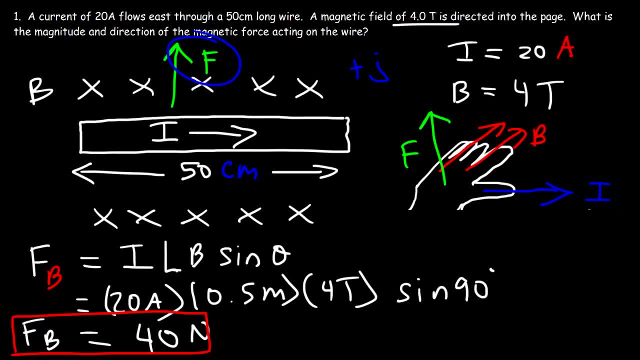 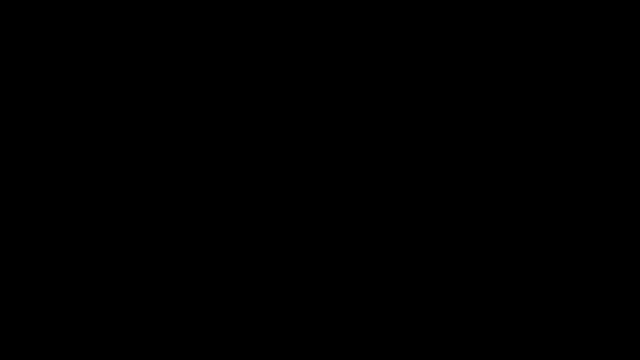 which is in the positive J direction. So you could say the magnetic field, or rather the magnetic force, is 40 J, if you want to write it that way. Now, for those of you who don't like to use the right hand rule, here is something that 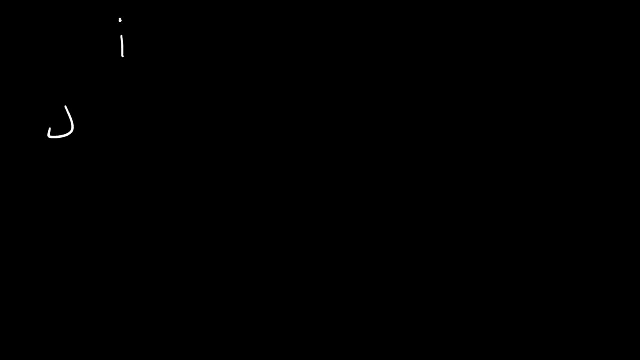 you can do So. let me give you a brief introduction into I, J and K. I represents the x values, So positive J represents the y values and K represents the z values. So let's say, if you want to find a cross product of I and J, 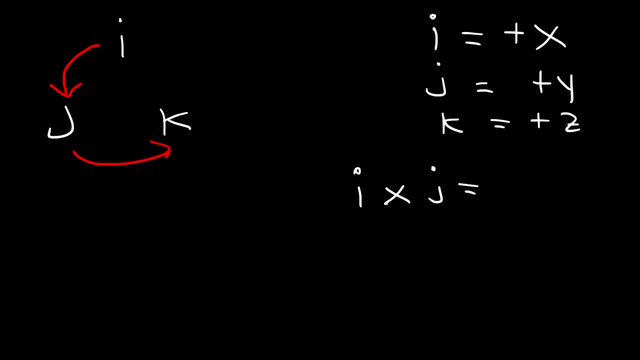 Start with I. I times the cross product of J is equal to K. Now, anytime you travel in this direction, that is, in the clockwise direction- Actually, that is counterclockwise- You're going to get a positive answer. If you travel in the clockwise direction, you're going to get a negative answer. 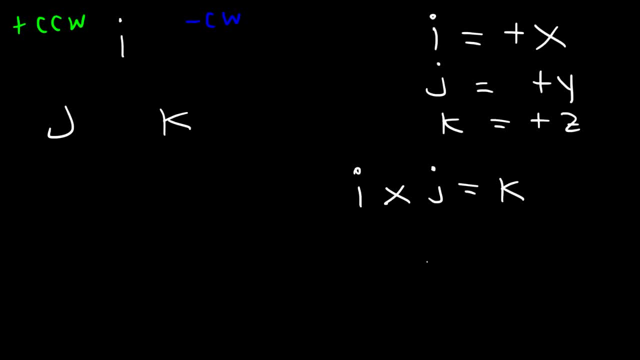 So keep that in mind. So let's say, if we wanted to find the cross product of J and K, So we're going to start with J, because it's on the left side. So the cross product of J and K is going to equal positive I, since we're moving in the 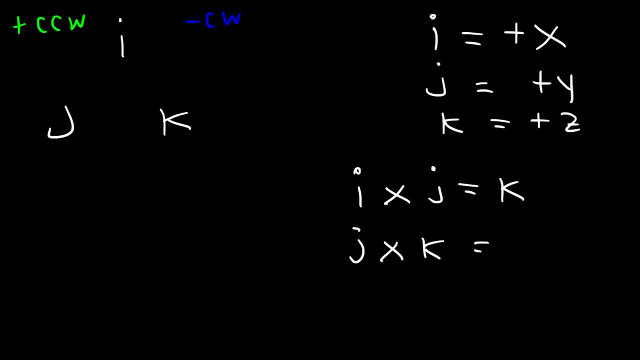 clockwise or the counterclockwise direction. I wrote that wrong. I meant to write that like this. Now let's say, if we want to calculate the cross product of I and K, So we're going to start with I and travel towards K. 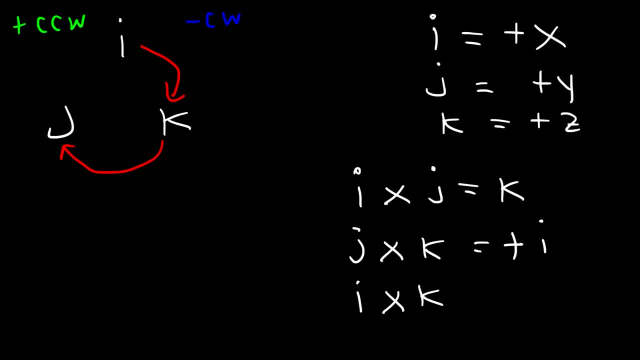 So the cross product of I and K is J. Now is it positive J or negative J? Now we're going in the clockwise direction as opposed to the counterclockwise direction, So this is going to be negative J. So try this one. 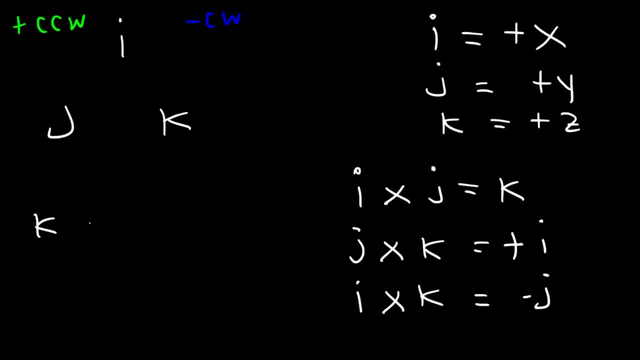 Actually, let me give you two problems: Calculate the cross product of K and I and also J, and I Try that. So if we start with K, go towards I, we're moving in the counterclockwise direction. So that's going to equal positive J. 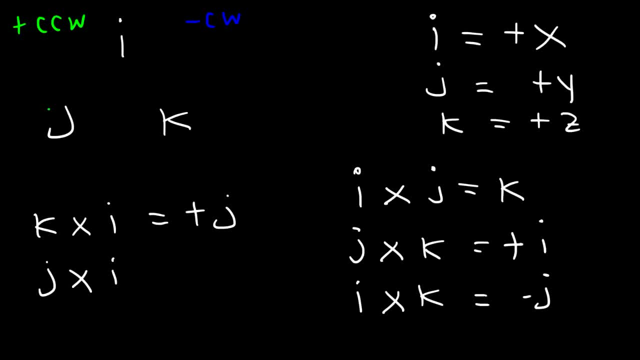 Now, if we start with J and we move towards I, we're going in the clockwise direction, So that's going to equal negative K. Make sure you understand that. Now let's apply it to the last problem. Let's see if we can get the same direction of the magnetic force acting on the wire. 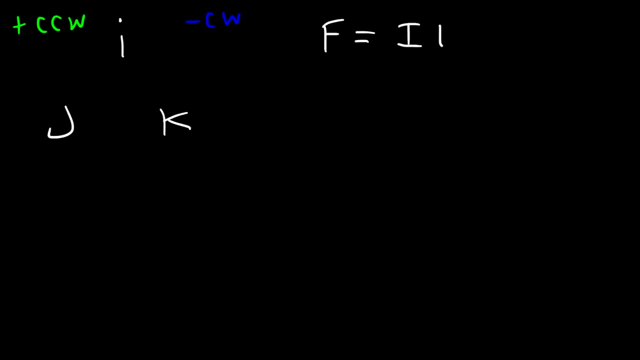 Now, the equation that we dealt with was: F is equal to ILB sine theta As a vector. The equation can be written this way: It's the current multiplied by the length of the wire times, the cross product of the magnetic field times sine theta. 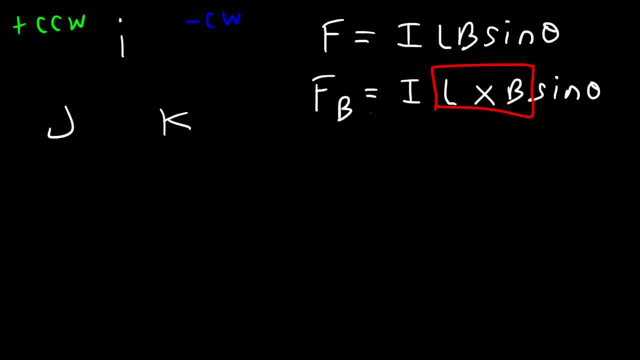 So let's focus on the cross product of L and B. So the length of the conductor is in this direction and the current in the conductor is flowing east. So we're going to start with this letter because that comes first And it's going in the positive X direction. 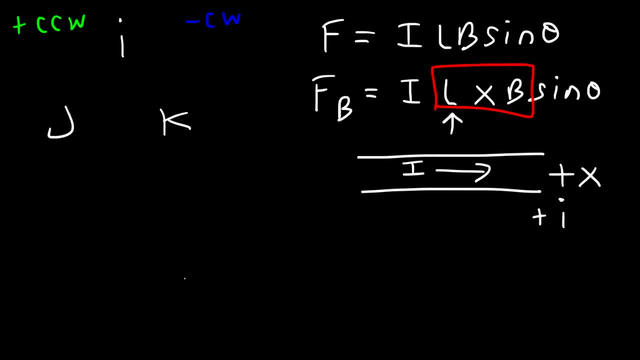 Which is associated with positive X. So we're going to start with this letter, because that comes first And it's going in the positive I. Now the magnetic field is directed into the page everywhere. So when you see this X symbol, it's into the page. 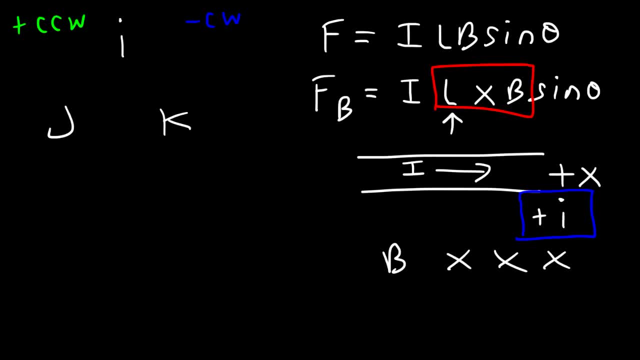 When you see a dot, that means out of the page. So because it's going into the page, that represents the negative Z direction, which is associated with negative K. So let's calculate the cross product of L and B. So basically, this is in the positive I direction or positive X direction. 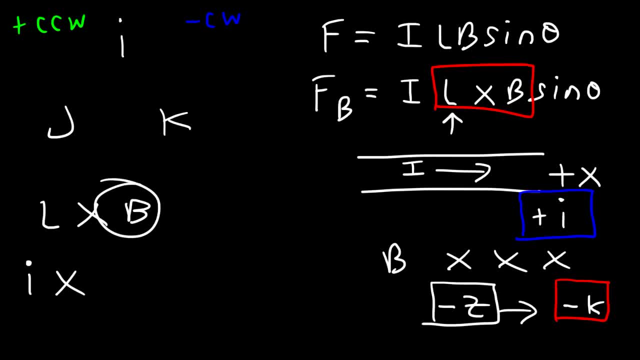 So that's just I And the magnetic field is in the negative K direction. So we need to find the cross product of I and negative K, But first let's find it for I and positive K. So, starting with I going towards K, this is going to equal J or negative J. 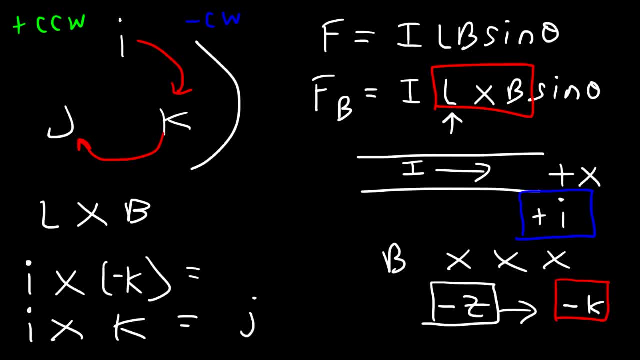 What would you say Now? because we're going in the clockwise direction. that's equal to negative J. So if the cross product of I and K is negative J, what do you think the cross product of I and negative K is going to be? 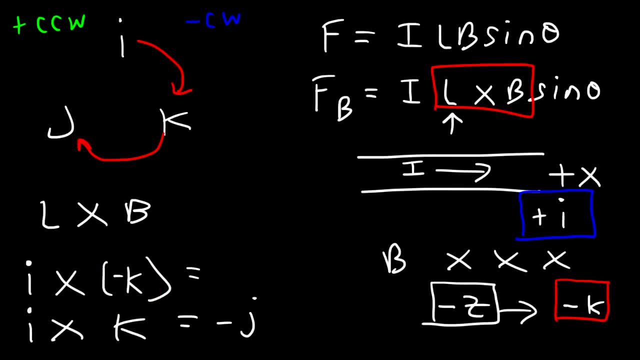 Well, if we add a negative sign, then this should change from negative J to positive J, And that's going to be the answer. So positive J represents the positive Y direction, And so that's what we have for the force. We said it was in the positive Y direction. 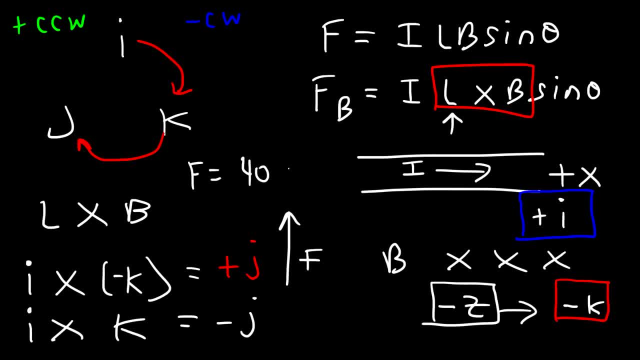 So you can write the answer as 40 Newtons and then times positive J. Now let me fix this J, It looks like an I. Now the 40 is the magnitude. J tells you the direction. So the magnetic force is 40 Newtons directed in the positive Y direction. 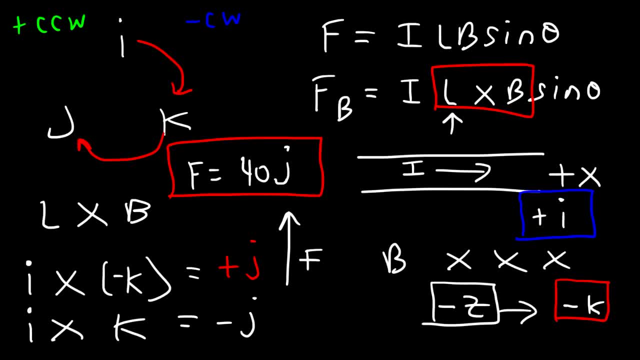 And so this is the technique that you could use to determine the direction of the magnetic force using the right hand rule. if you don't want to use the right hand rule, if you want to use I, J and K, But you need to know the formula as a vector. 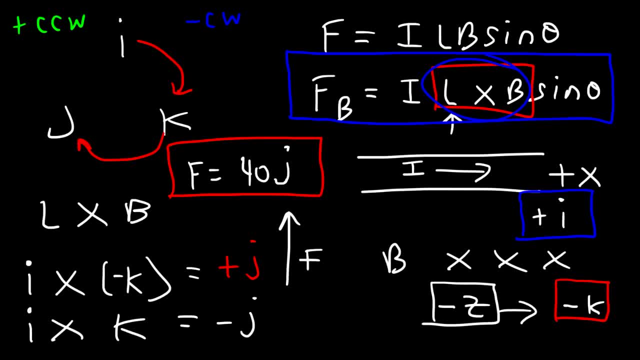 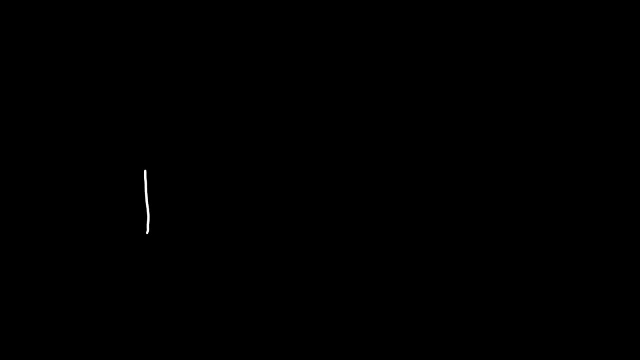 Because the order in which this is written is very, very important. For example, B cross L will give you a completely different answer than L cross B. So that's why the direction, the order in which you do it, matters. Now, let's say, if we have a conductor with a current flowing in this direction. 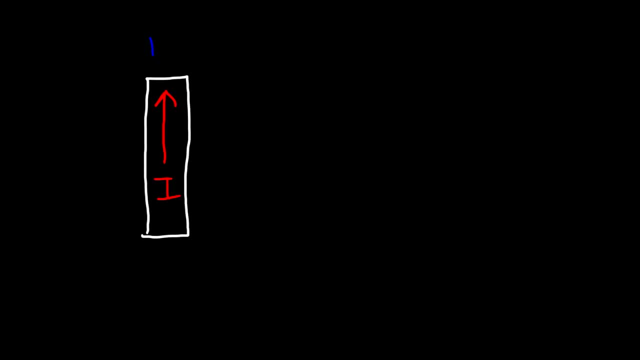 So the current is flowing in the positive Y direction. So the current is flowing in the positive Y direction, So the current is flowing in the positive Y direction And, let's say, the magnetic field is in this direction, So it's directed in the positive X direction. 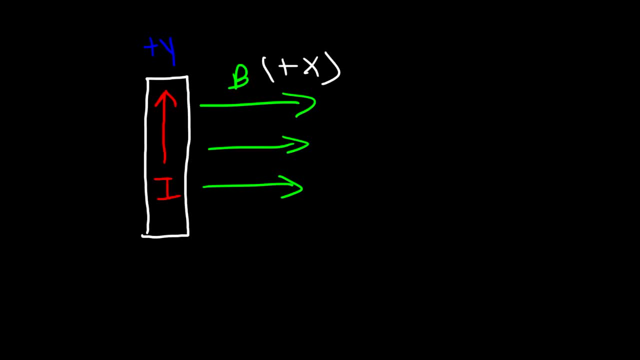 What is the direction of the force? Now, if the magnetic field is in the X direction and if the current is in the Y direction, the magnetic force has to be in the Z direction. either positive Z or negative Z. It's either into the page or out of the page. one of those two answers. 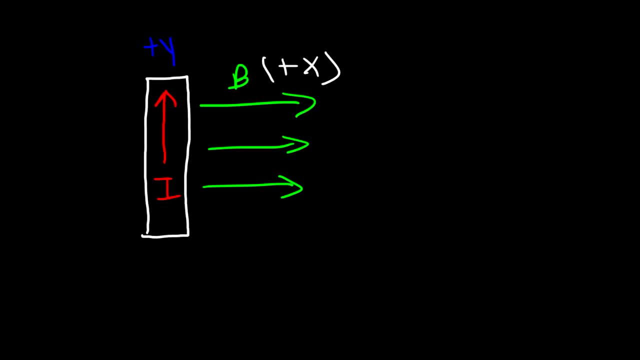 Now let's use the right-hand rule first to get the answer. So what you need to do is you want to point your thumb in the direction of the current and your four fingers in the direction of the magnetic field. If you do that, notice that the palm of your hand should be pointing into the page. 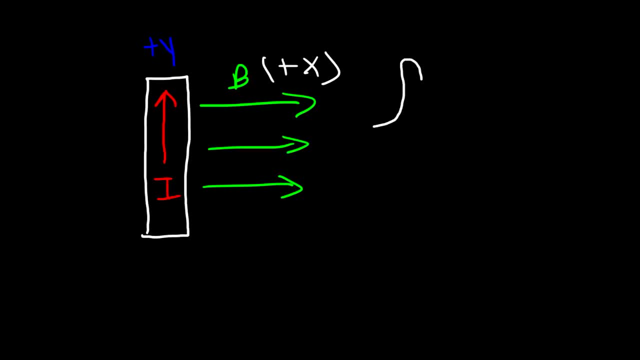 So let's see if I can draw that. So we want the thumb to be in the direction of the current and your four fingers to be in the direction of the magnetic field. So I'm going to draw that. So we're going to draw the thumb. 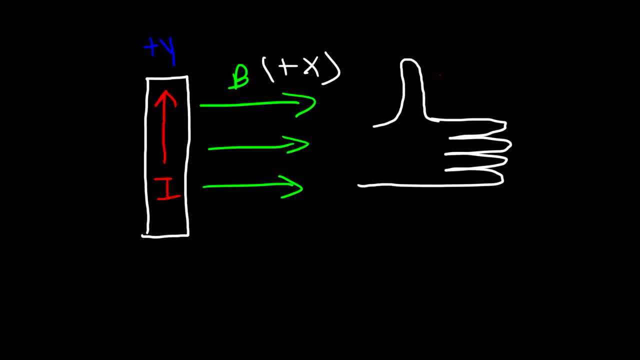 So this is the current- Let's use a different color- And this is the direction of the magnetic field. So the force which comes out of the palm of your hand is going into the page, And so we can represent that with an X symbol. 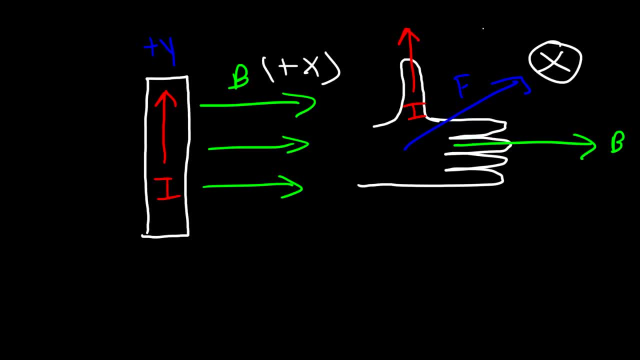 So therefore, because it's going into the page, it's going in the negative Z direction, which is equivalent to negative K. Okay, Now let's get the same answer using the other technique. So this is going to be I, J and K, in that order. 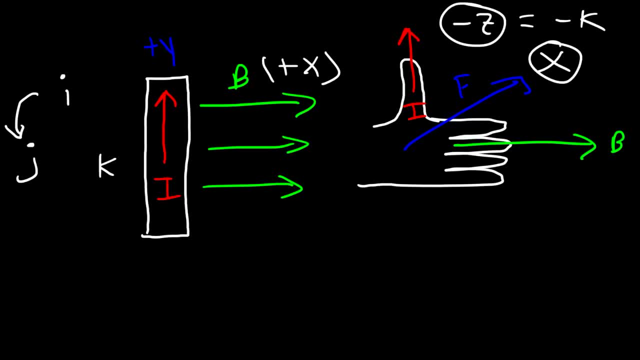 And remember, if you're going in the counterclockwise direction, it's positive And if you're going in the clockwise direction, it's going to be negative. So we need to focus on L, cross B, So L and the direction of the current is going to be the same. 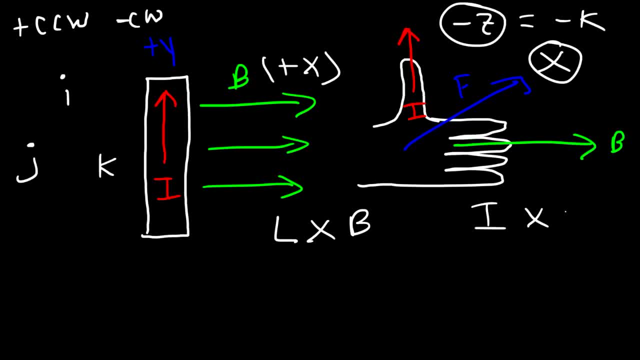 So you can think of it as the current times or the cross product of the current and the magnetic field. You can do it in that order. You should get the same answer. So the current is flowing in a positive Y direction. So positive Y is associated with positive J. 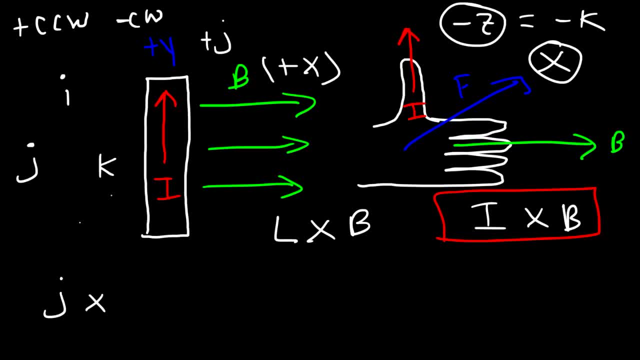 So we have J and the magnetic field is going in the positive X direction. So that's positive I. So we need to find the cross product of J and I. So start with J and go towards I And then keep going. So this is going to give us K. 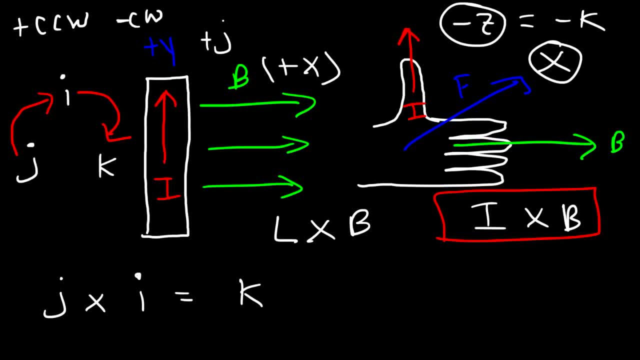 Now, is it positive K or negative K? Are we moving in the clockwise direction or the counterclockwise direction? Notice that we're moving in the direction of a clock, So this is clockwise, which is going to give us a negative sign. 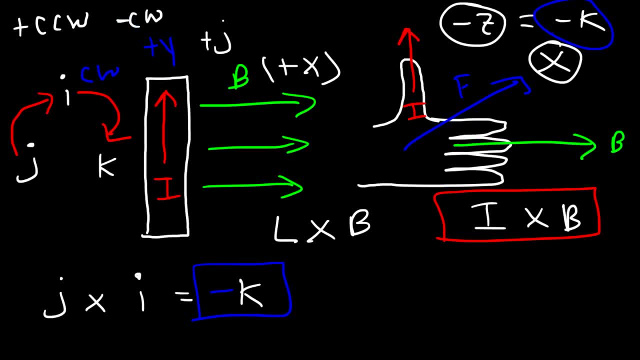 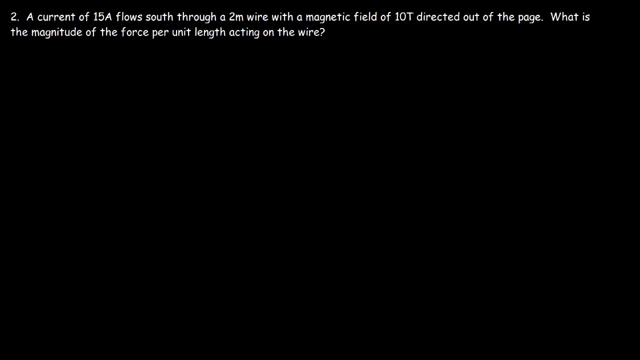 So this is going to be negative K, which is in agreement with what we have. So now you have two ways to determine the direction of the magnetic force acting on a current-carrying wire or a current-carrying conductor. Number two: a current of 15 amps flows south through a 2-meter wire. 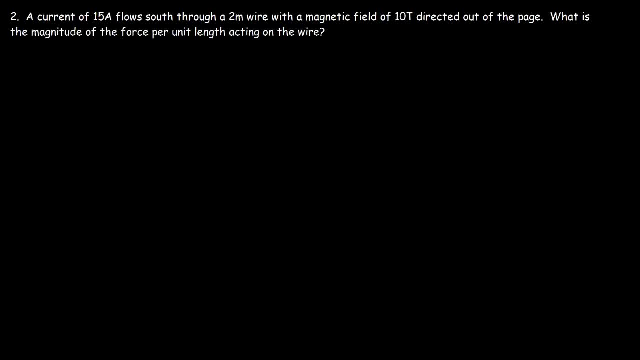 with a magnetic field of 10 Tesla directed out of the page, What is the magnitude of the force per unit length acting on the wire? So let's draw a picture. So let's say: this is the wire and we have a current. 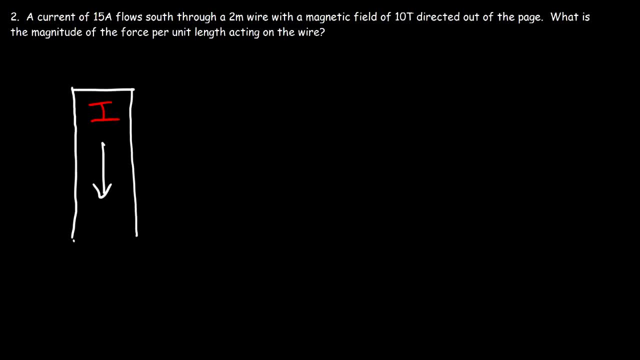 It's flowing south in it. So the current is in the negative Y direction, or we could say negative J. The magnetic field is directed out of the page. So the magnetic field is in the positive Z direction, or positive K. Now where is the magnetic force? 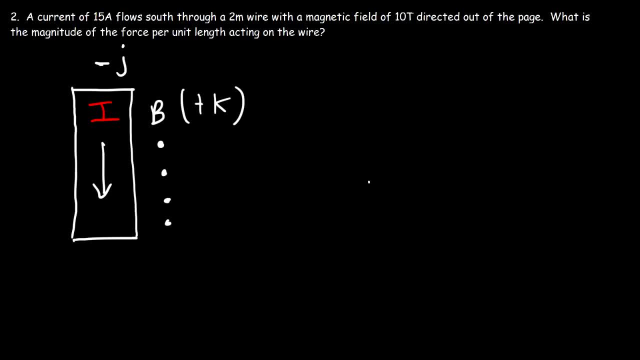 So if we draw a picture, we need to point the thumb in this direction. That is this direction. So the magnetic field is going south and the four fingers have to be going out of the page. So just work with it, John. 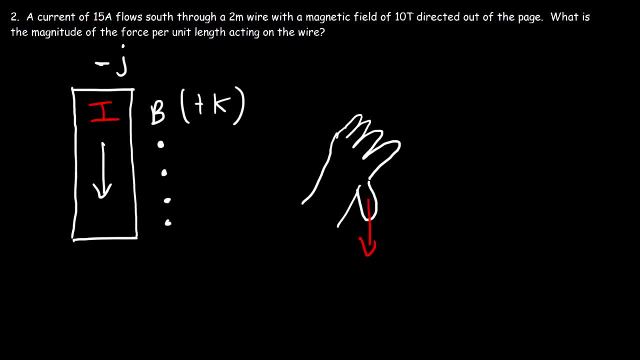 I know it's not ideal, but make the best of it. So this is the current, and here we have the magnetic field going in this direction. So the force is going to be coming out of the palm of your hand and so it's going to be going west. 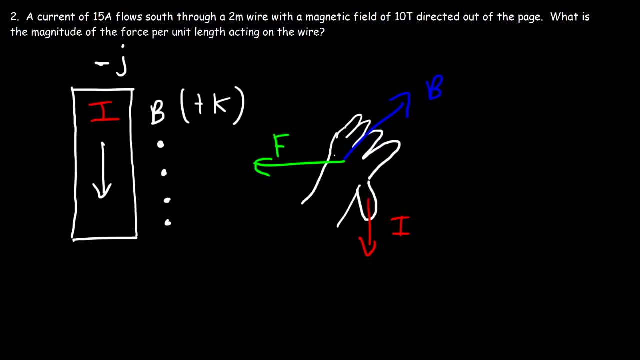 And right now, each of these, Each of these values are perpendicular to each other, So we have the magnetic force going in this direction. So west is negative X, which is negative I. So let's confirm that answer using the other technique. 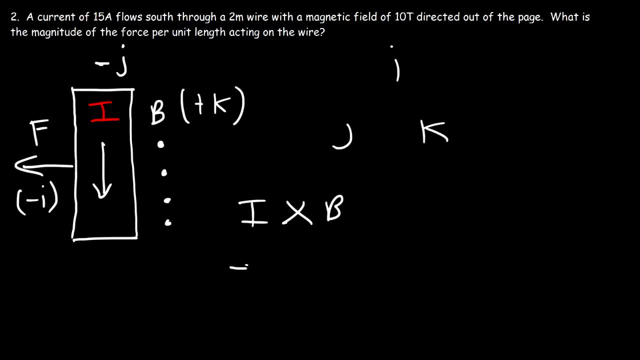 So I cross B. The current is in the negative J direction And the magnetic field is in the positive K direction. So first let's find the cross product of J and K. So starting with J, let's go towards K And that's going to equal I. 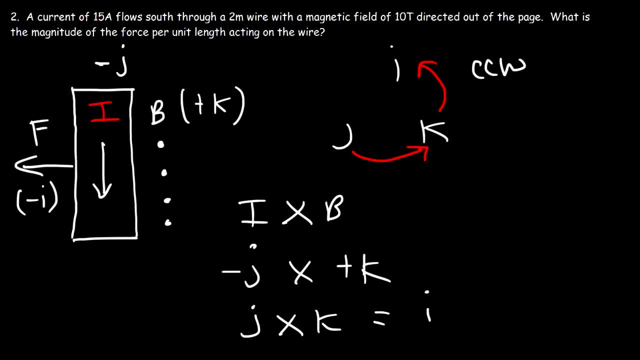 Now we're going in the counterclockwise direction, so that's going to give us a negative answer, Actually a positive answer. Clockwise is negative, So this is going to be positive I. So negative J cross, K, K has to be negative I. 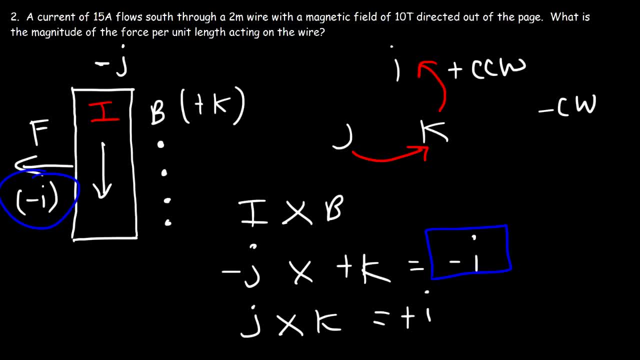 And so that is an agreement with the answer that we have. So negative I is left or in the negative X direction, which is west. Now let's finish the question. So we need to calculate the force per unit length. F is equal to ILB sine theta. 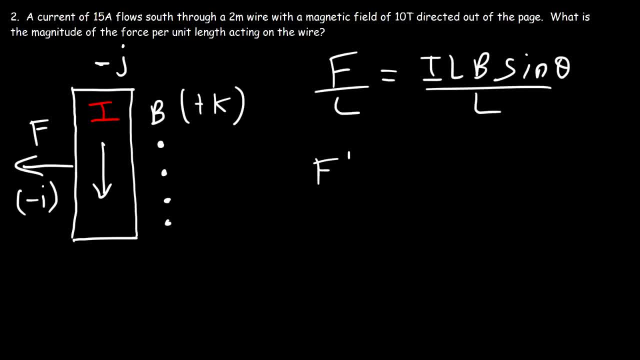 So let's divide both sides. So the force per unit length F over L is going to equal the current times, the magnetic field times sine theta. So the current is 15 amps, The strength of the magnetic field is 10 Tesla. 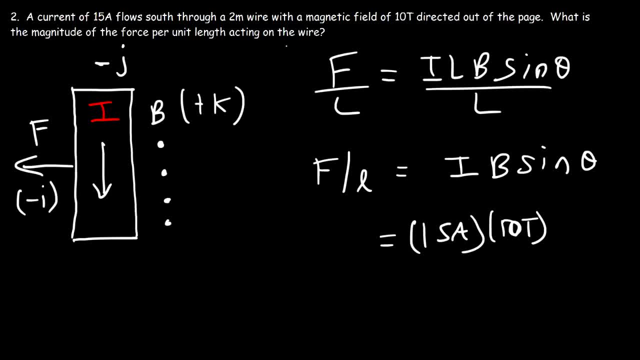 And the angle between the magnetic field and the current is going to be 90. This is in the Z direction, That's, in the Y direction or the negative Y direction. So sine 90 is 1.. So it's simply 15 times 10.. 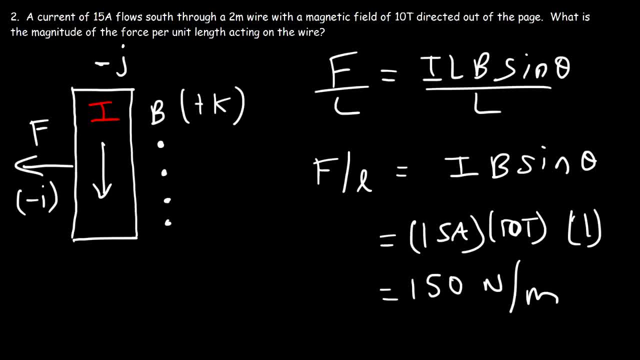 So it's going to be 150 newtons per meter. So that's how you can calculate the force per unit length acting on the wire. So what is the force acting on 2 meters? This tells us the force that acts on 1 meter of the wire. 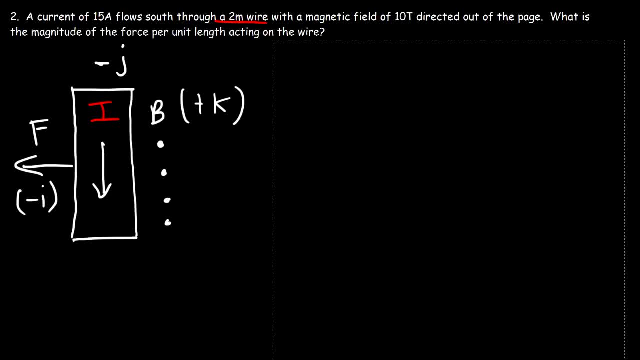 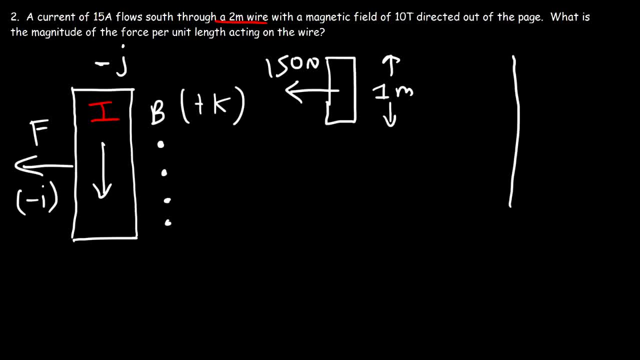 Now if we double the length, let's say if we make it 2 meters long, the force is going to double. So it's going to be 300 newtons, because 300 divided by 2 will still give us 150 per meter ratio. 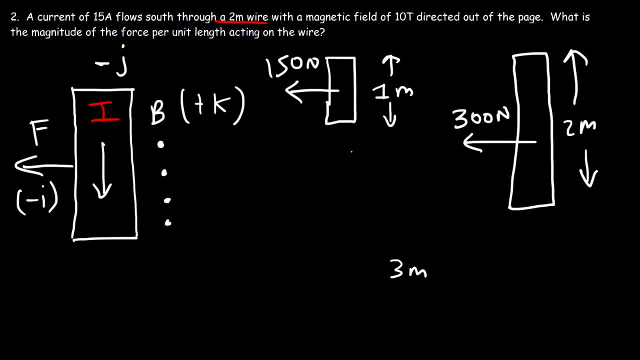 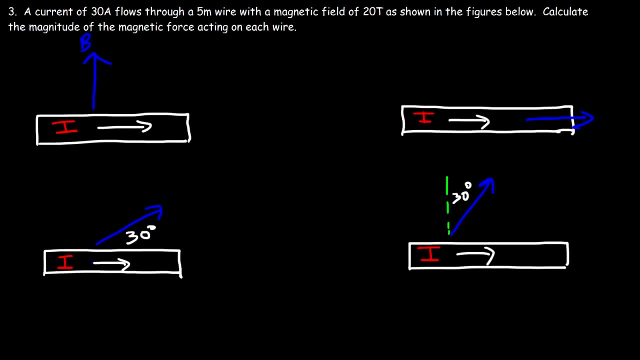 So if we triple the length, let's say if we make it 3 meters, then it's going to be 150 times 3.. So the magnetic force is now 450 newtons. Number three: a current of 30 amps flows through a 5 meter wire with a magnetic field of 20 Tesla, as shown in the figures below. 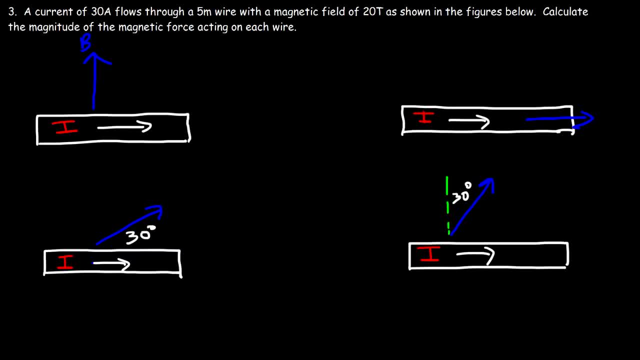 Calculate the magnitude of the magnetic force acted on each wire. So let's not worry about the direction in this problem. So notice that the current and the magnetic field are perpendicular to each other, So therefore the angle that we need to deal with is 90.. 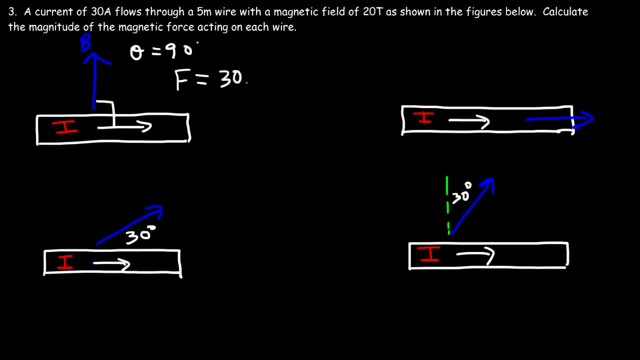 So it's going to be I L B. The current is 30 amps. Let me see if I can put that below the wire, And then the left of the wire is 5 meters times the strength of the magnetic field, which is 20.. 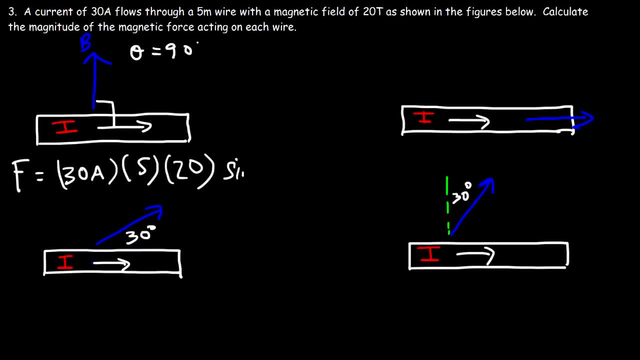 And then times sine of 90. So 30 times 5 times 20. That's 3000 times sine 90. So the magnetic force is going to be 3000 newtons in this case. So that's it for the first part. 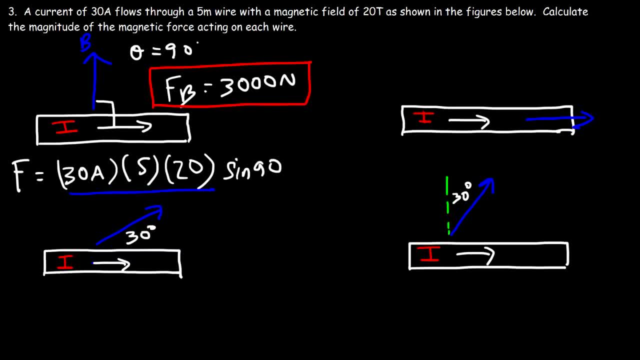 Now these three numbers won't change. So for the second part it's going to be 30 times 5 times 20, which is 3000.. But what's the angle in this example? Notice that the current and the magnetic field are parallel to each other. 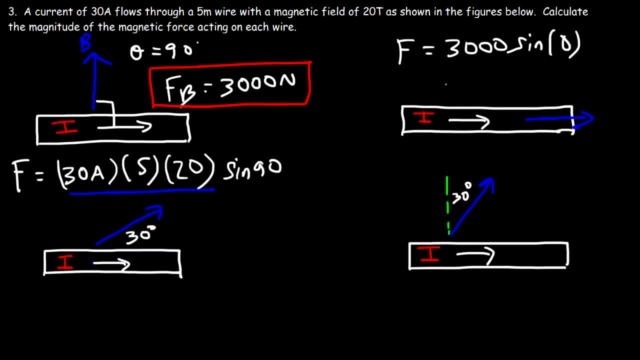 So therefore the angle is zero. Sine zero is one. So the magnetic force is zero. Whenever the current is parallel to the magnetic field, the magnetic field does not exert a force on that current. It has to be perpendicular or at an angle. 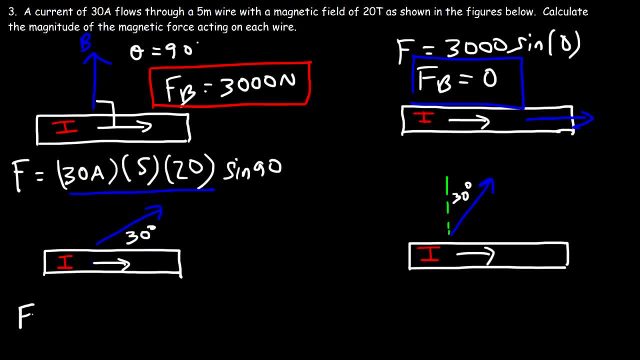 Now let's move on to the third example. So I L B once again, is 3000.. Now the angle between the current and the magnetic field, as you can see, it's 30 degrees. So this is going to be sine 30 and sine of 30 degrees is one half. 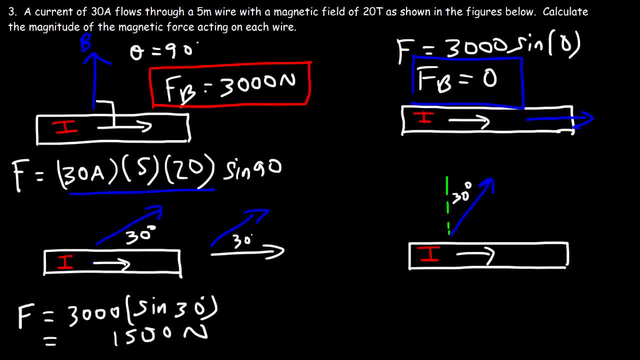 So half of 3000 is 1500. And so that's the magnetic force acting on the wire in this case. Now for the other example. you need to be careful. the angle between the normal line with respect to the normal line. The angle between the normal line with respect to the normal line with respect to the normal line with respect to the normal line. 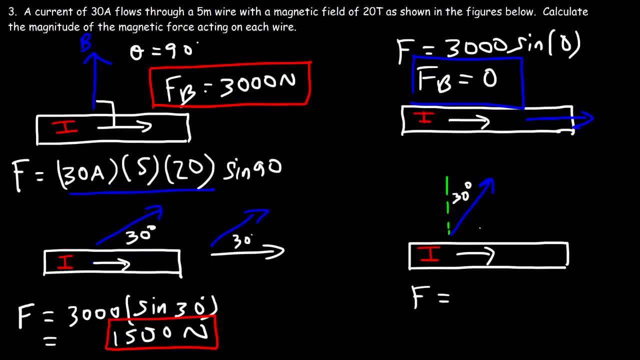 The angle between the normal line with respect to the conductor and the magnetic field is not the one you want to use. You need to use this angle 60. So it's I L B 3000 times sine of 60. And so that comes out to be 2598 newtons.